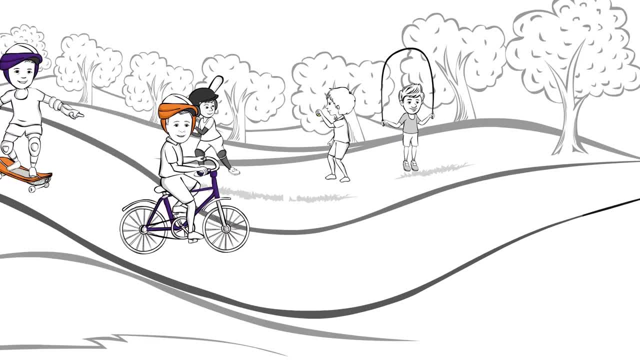 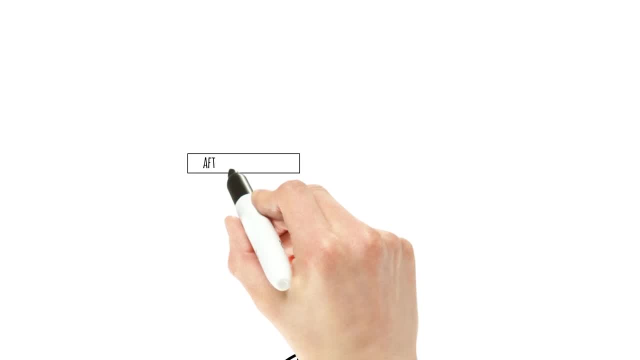 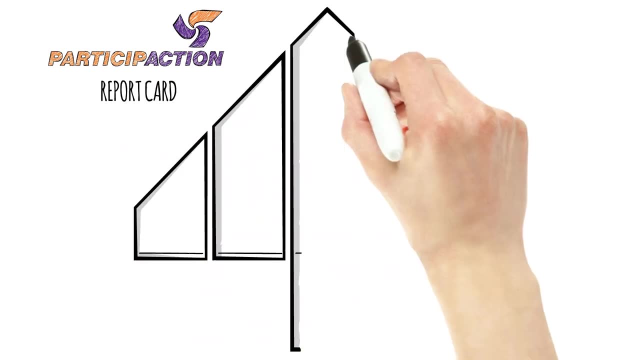 You probably already know a child who is physically active has better heart, muscle and bone health. But did you also know that physical activity boosts brain health in kids too? That's right. The 2018 Participation Report Card on Physical Activity for Children and Youth. 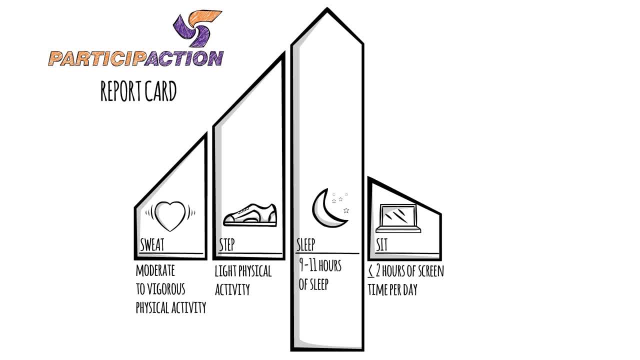 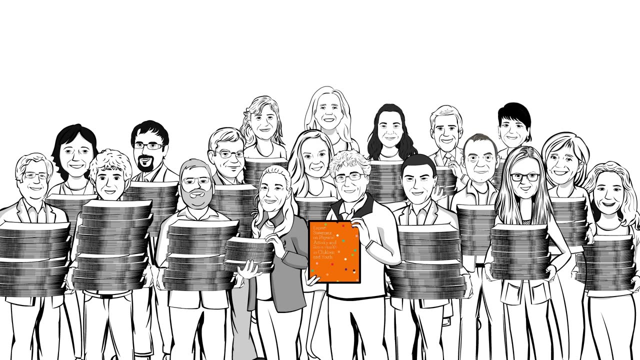 reports that kids who meet the physical activity recommendations within the Canadian 24-Hour Movement Guidelines have better cognition, brain function and mental health. Participaction and an expert panel of neuroscientists, exercise scientists and disability specialists reviewed hundreds of studies. 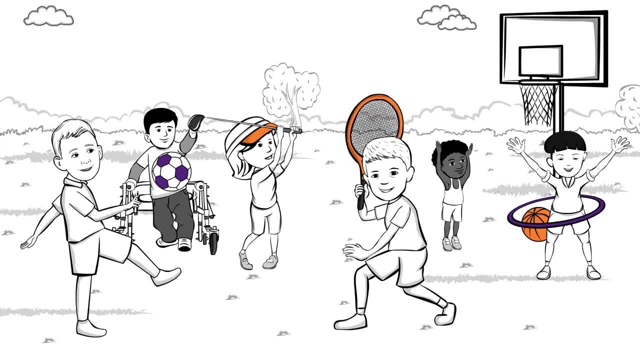 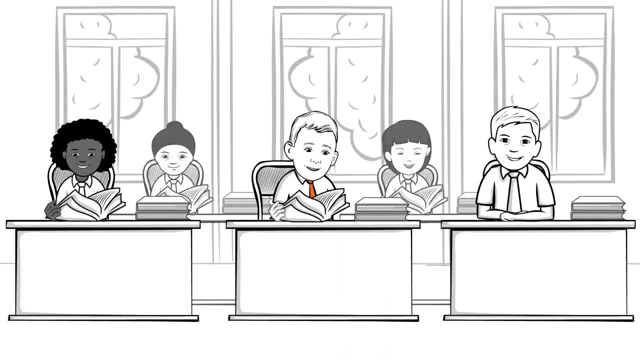 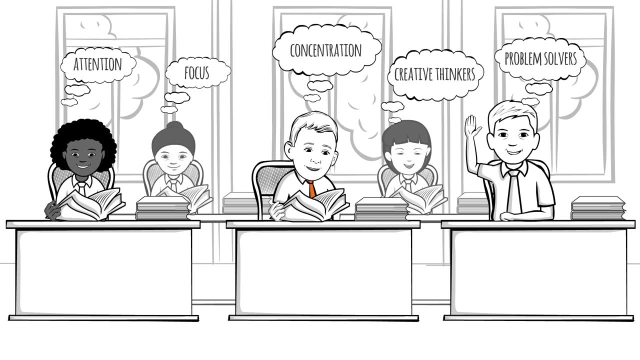 We found that children who are physically active have better performance in math, reading, science and social studies. These kids also have better attention, focus and concentration. They are better creative thinkers And better problem solvers. In fact, these active kids have even larger brains. 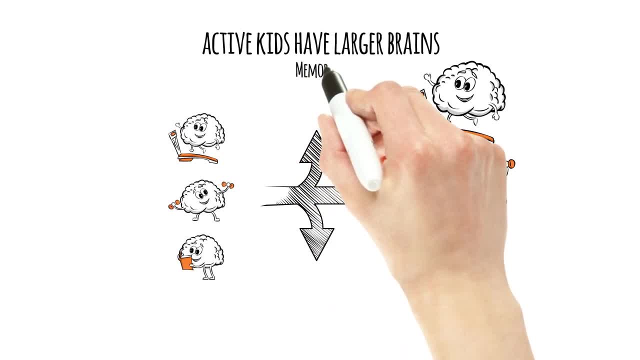 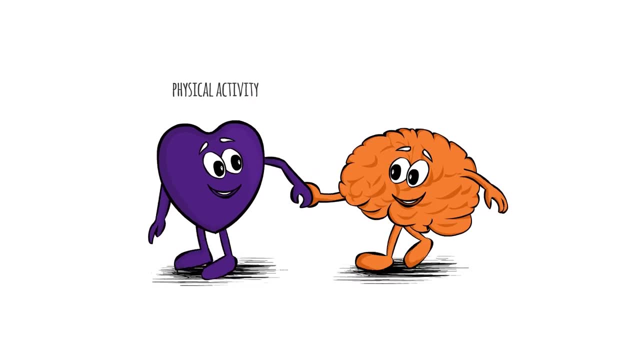 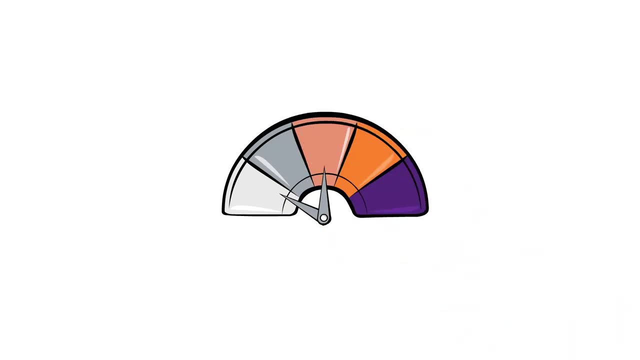 Especially in the areas of the brain related to memory, higher level thinking and emotion. This leads us to another important benefit of physical activity in children and youth: Better mental health. Active kids have fewer depressive symptoms, feelings of anxiety and overall they just feel happier. 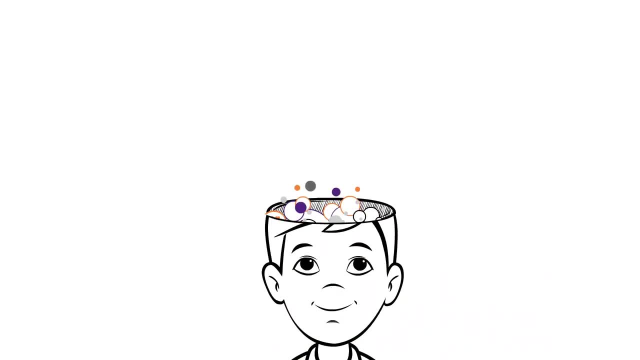 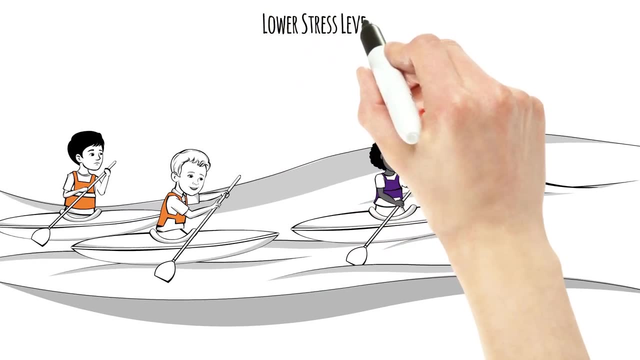 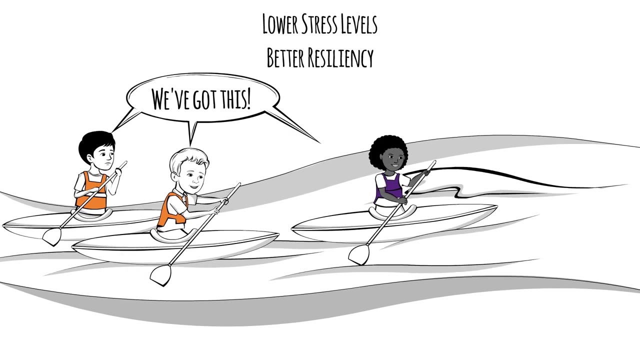 More specifically, research suggests that the brain releases these feel-good chemicals when children are getting active. Physical activity is associated with lower stress levels and better resiliency, particularly in the teen years. Self-esteem, self-concept and self-worth are all improved in active kids. 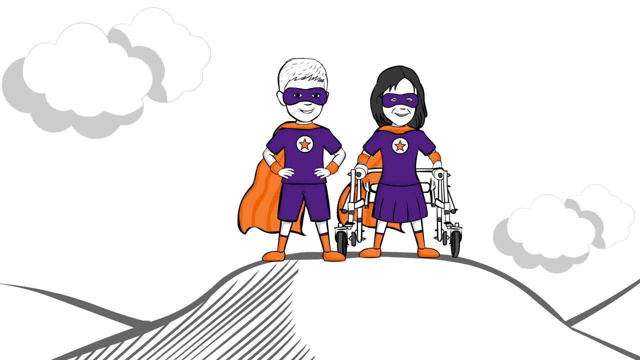 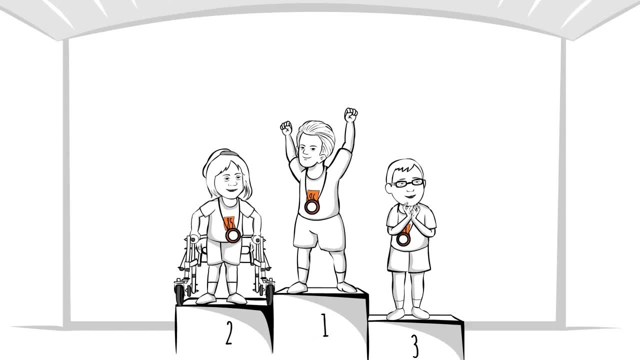 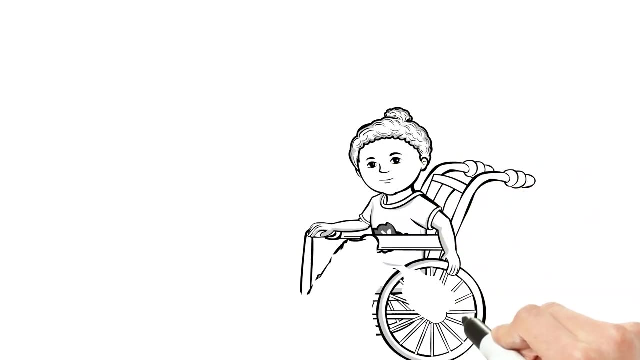 Now this doesn't just apply to typically developing children. Importantly, many of these benefits are also reported in children with disabilities. In fact, Kids with disabilities may experience different cognitive habits, experience even greater gains by increasing their activity level. Now, unfortunately, we know that. 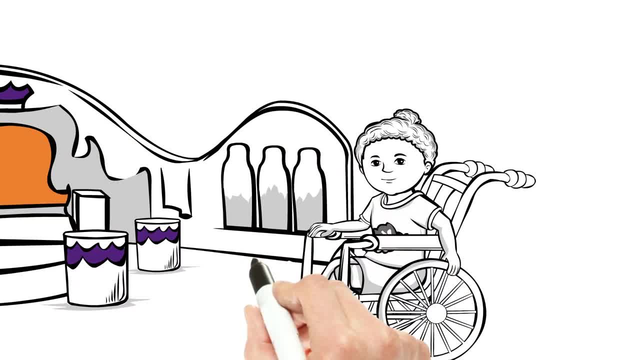 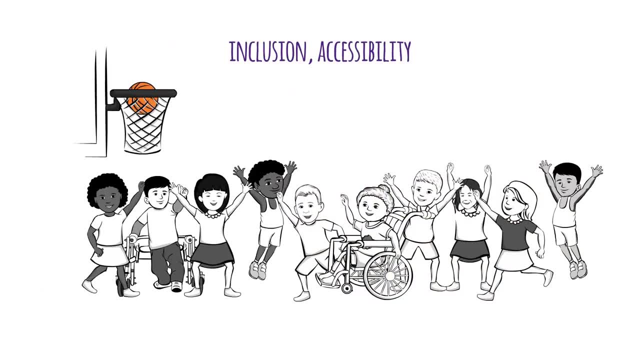 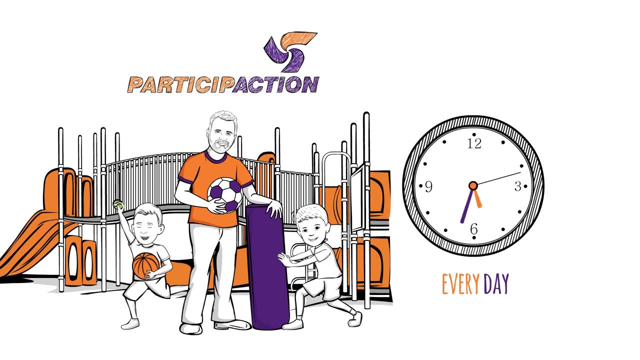 kids with disabilities often experience more barriers to being active and are generally less active as a result. For that reason, inclusion and accessibility for kids with disabilities is really important. So if you're a parent, educator, healthcare provider or coach, I want you to ask yourself: how can I encourage a kid to get active for 60 minutes today? 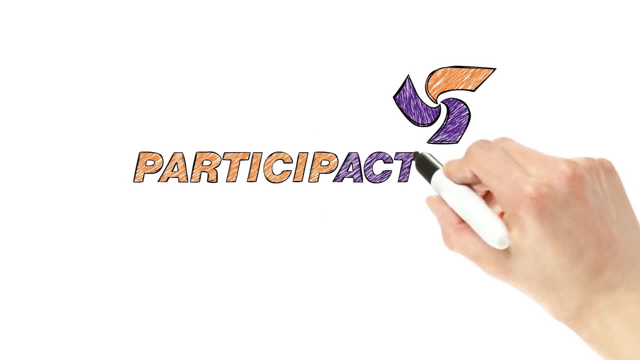 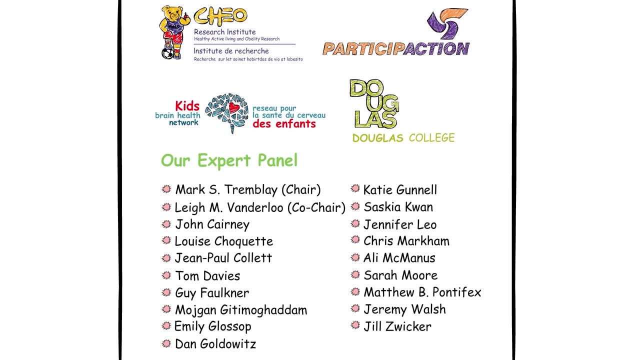 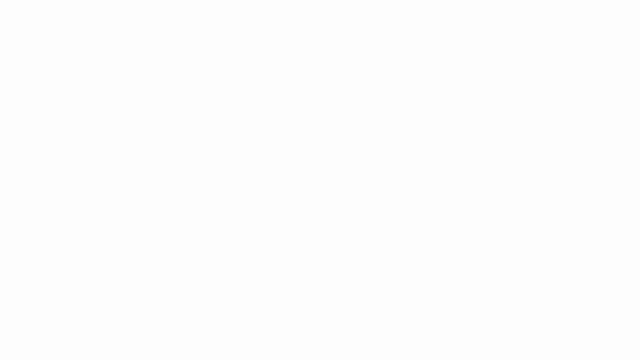 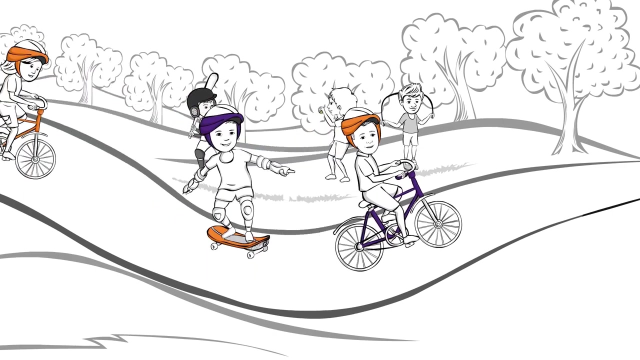 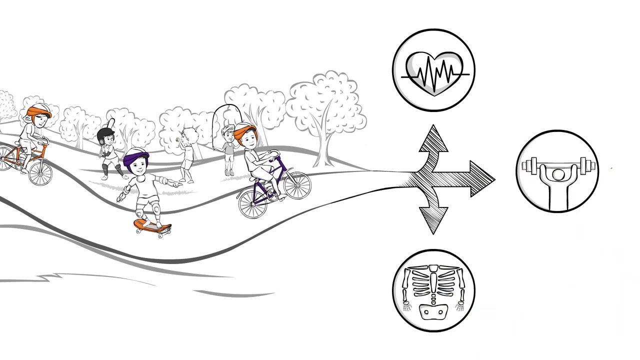 and every day. Visit participationcom forward slash report card to learn more. A child who maintains a good level of physical activity enjoys better health at heart, muscles and nose. But did you know that physical activity also improves the health of the children's? 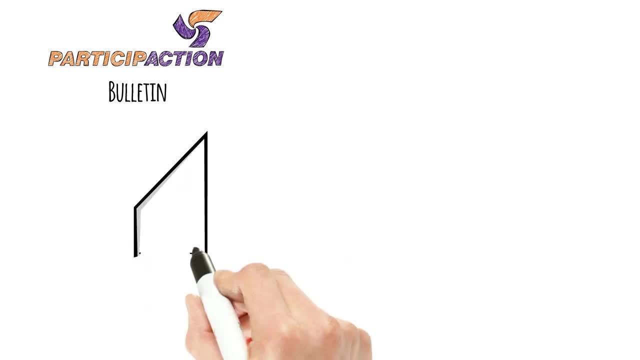 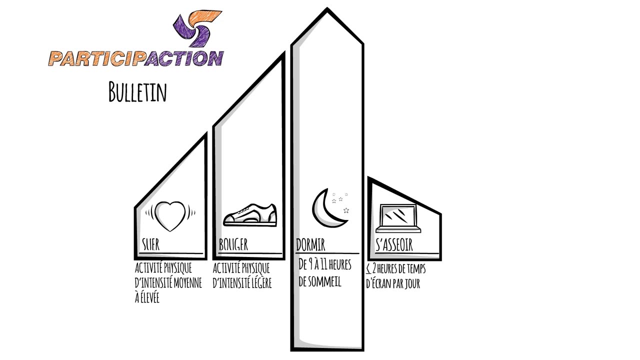 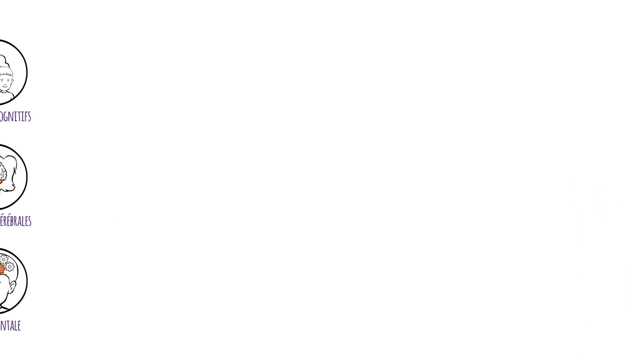 brain. In fact, the physical activity bulletin for participating children reveals that children and young people who follow the recommendations of the Canadian Directive on 24-hour movement benefit from better cognitive processes, brain functions and better mental health. With a committee of experts, we can help you improve your physical and mental health. 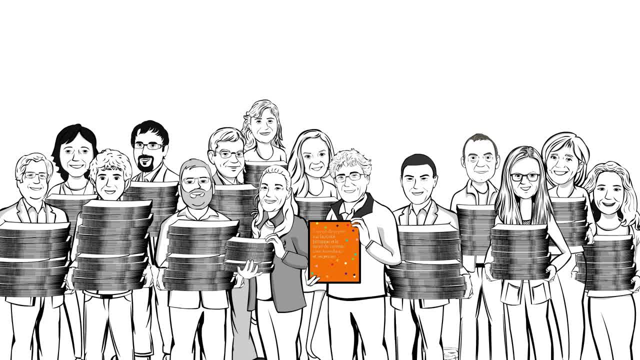 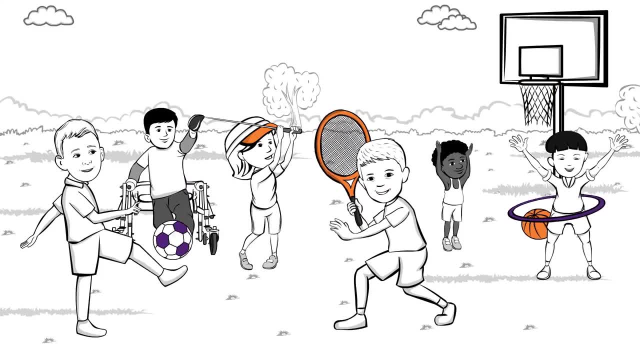 In addition to studying neuroscience, physical activity science and accessibility, specialists Participation has reviewed hundreds of studies. We have discovered that children who do physical activity get better results in mathematics, reading, pure and social sciences. These children are also more attentive and show better concentration. They develop their creative thinking and problem-solving. 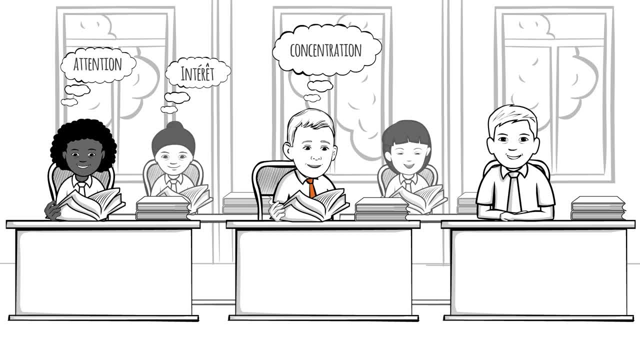 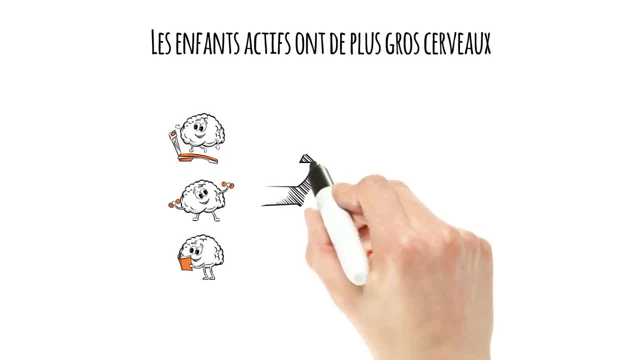 skills more. In fact, these children even have bigger brains, especially in the areas of the brain linked to memory. In addition, they have a better ability to read and write and write. In addition, they have a better ability to write and write. In addition, they have a. 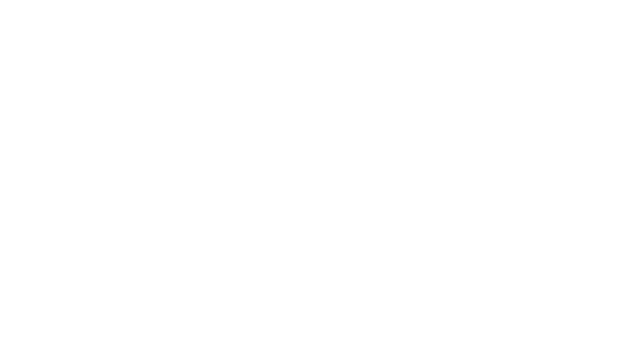 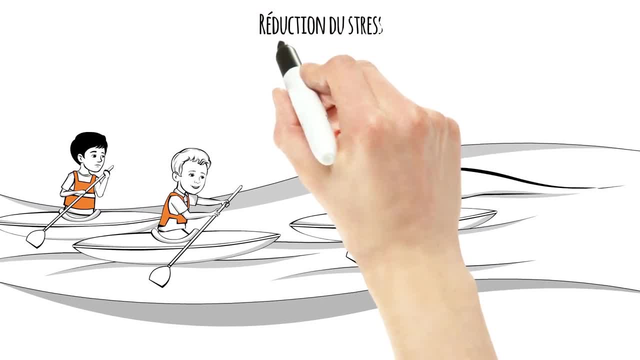 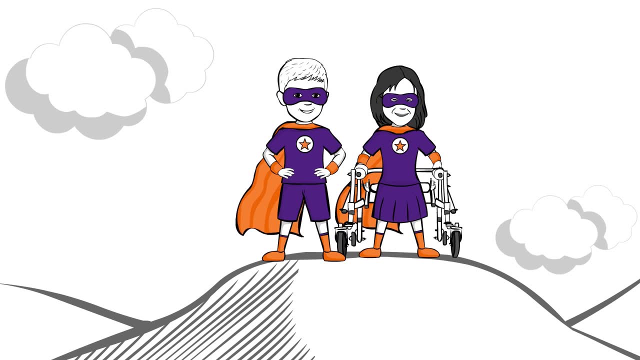 and diagnosis and sessions can have better results without abuse. How many childrenática are there in Canada, I'll tell you- are more confident and feel more valued. Moreover, this does not concern children with normal development. It has been shown that children with an imitation also benefit from these benefits. 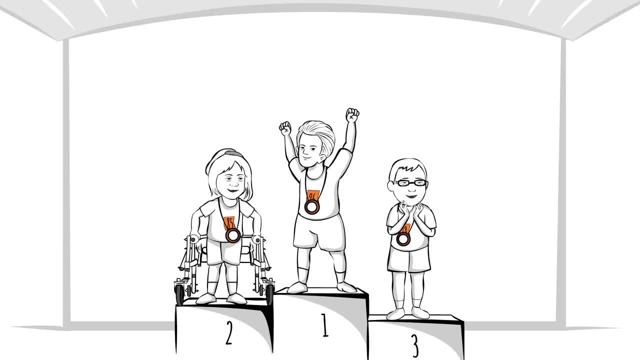 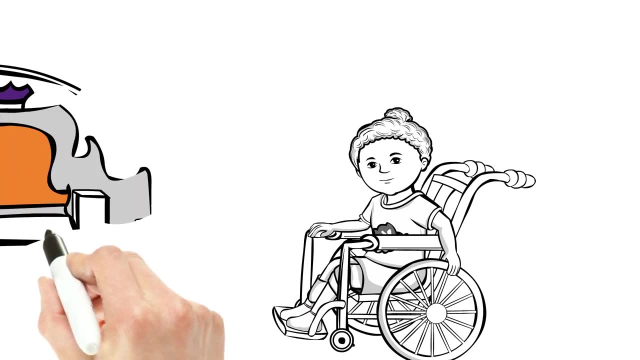 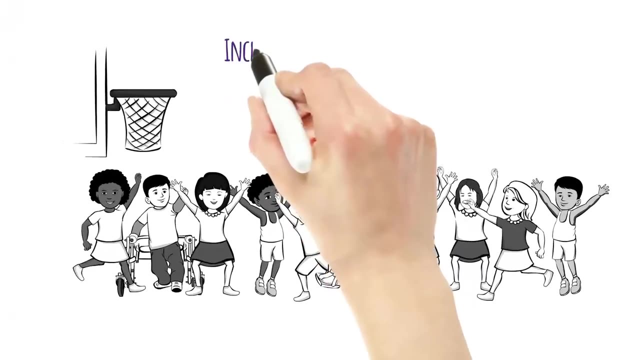 Children and young people with an imitation could even gain greater benefits from increased level of physical activity. Unfortunately, we are aware that children with an imitation must overcome many obstacles to physical activity and, consequently, are often less active than their father. For this reason, it is important to ensure inclusion.